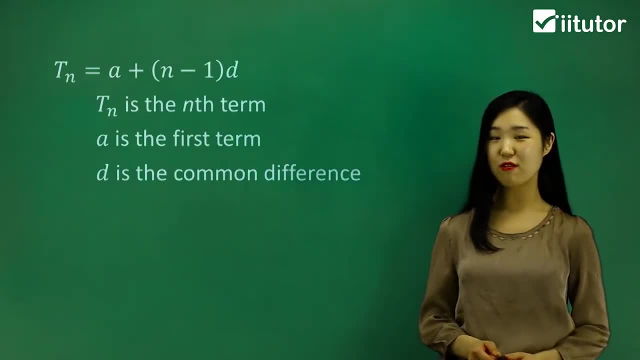 Let's look at some application questions. using arithmetic sequence. And you know that this is the formula that we're going to be using, the TN formula, where TN is the nth term. So make sure you remember this, guys. TN is A plus N minus 1D, And you know that A is the first term, D is the common difference, right? So let's use that to try some application questions. I'm going to go straight into question one. Let's read it together, guys. 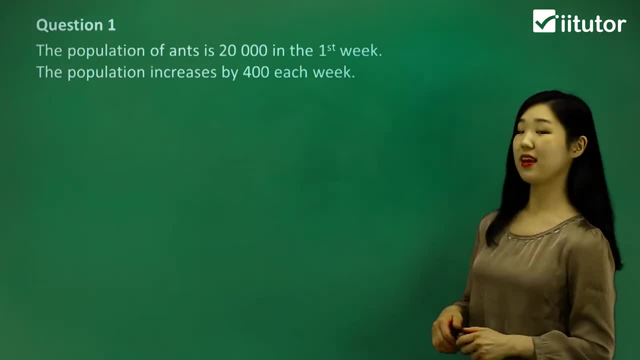 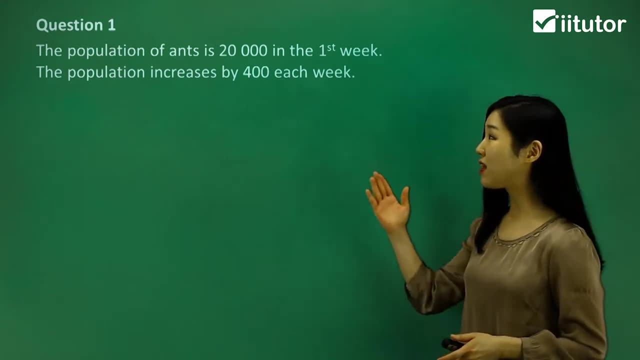 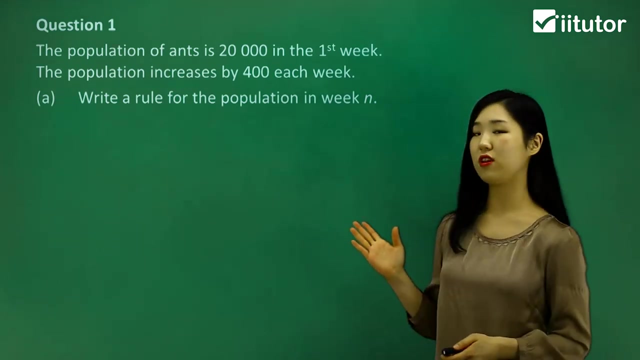 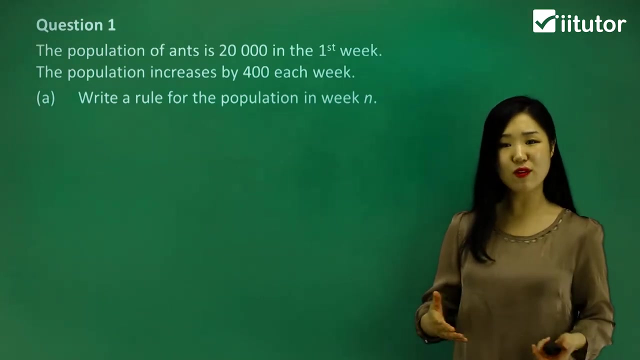 It says the population of ants is 20,000 in the first week And the population increases by 400 each week. So you can see that we begin with 20,000.. Now we're going to be first finding the rule, So write the rule for the population in each week: N. So we want to keep it in terms of N, but we want to write a rule for it using our arithmetic sequence, And it's definitely going to be arithmetic, isn't it? Because it tells us that it increases by the same number, 400,. 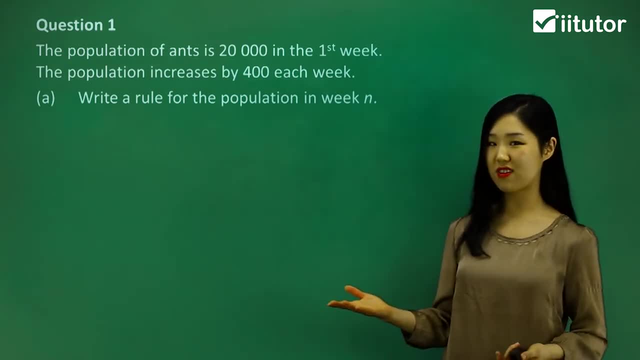 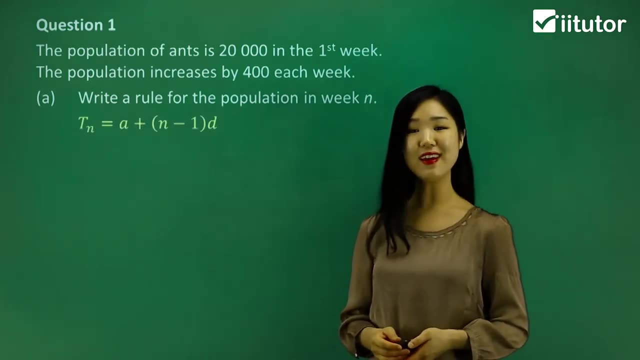 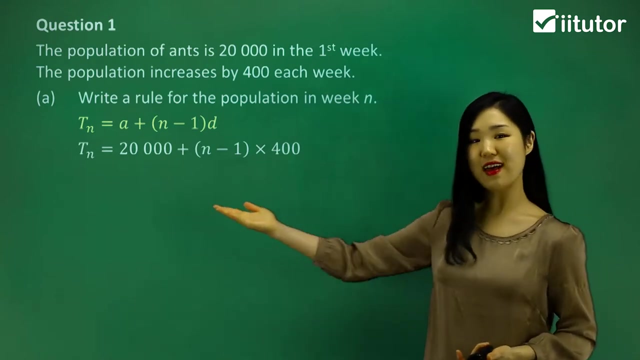 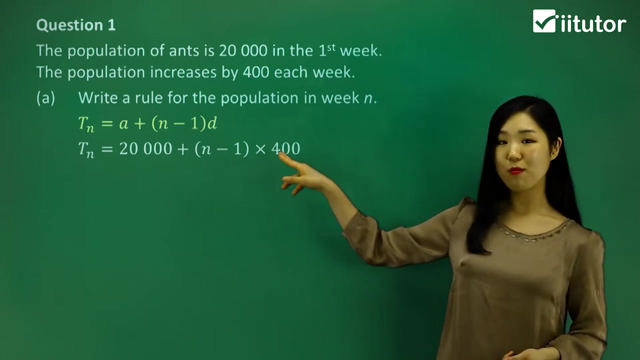 each week, And that kind of links us with the common difference. You can see that the common difference is probably just 400, isn't it? So we're going to be using our formula: TN equals to A plus N minus 1D. And, guys, the first term is 20,000.. See, it starts with 20,000 in the first week, So that's the first term A, So 20,000 is going to be your A. And see how I replaced the D with 400?, Because I've mentioned that 400 was the common difference. Every single week it increases by 400.. 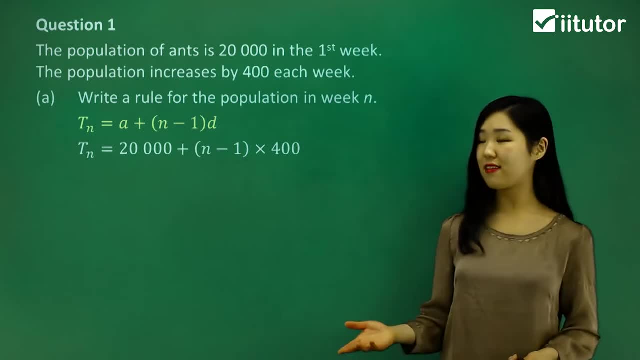 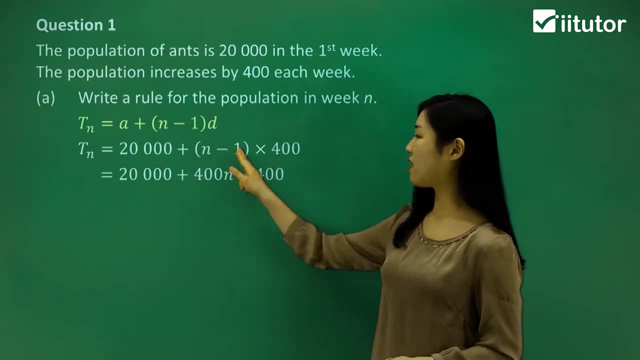 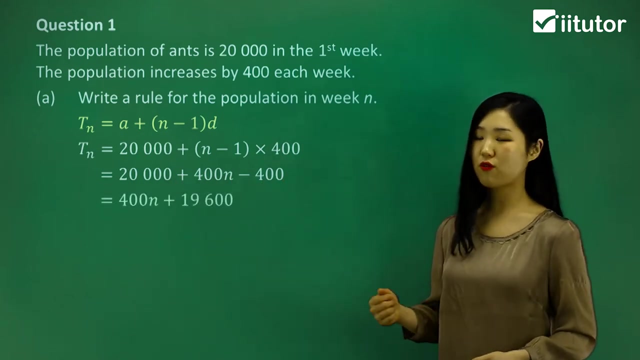 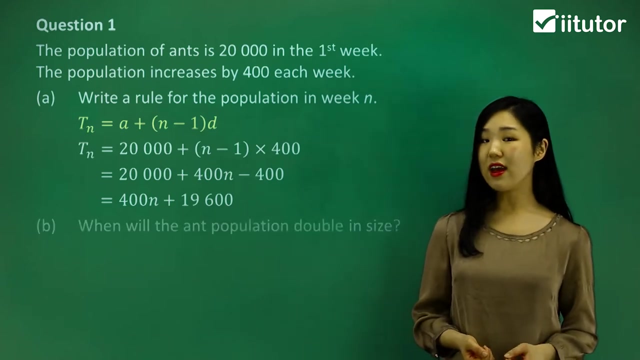 So that's going to be the common difference. So now, guys, let's just expand and simplify it and find the final rule. So I've expanded the brackets 400 times N is 400N, That's going to be 400. And then you can see that 20,000 minus the 400 will give us 19,600. So it's just 400N plus 19,600. That's just our rule. We can't simplify that any further. So that's the rule for TN. Now what we're going to do in part B is asking us: when will the ant population double in size?